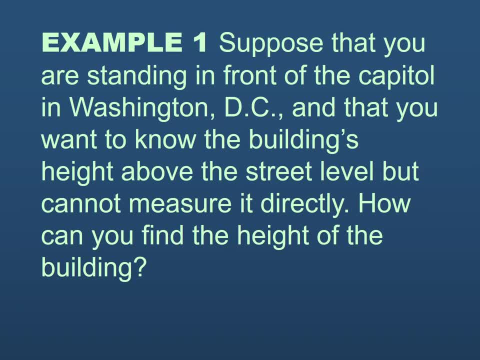 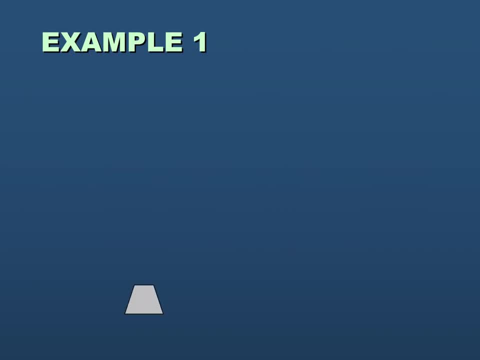 just take a measuring tape up to the building. We want to try to find the height of the building, Okay, so here's a diagram that we can make here. Okay, Alright, let's say that this distance is 345, and this distance is 6, and we are 5. 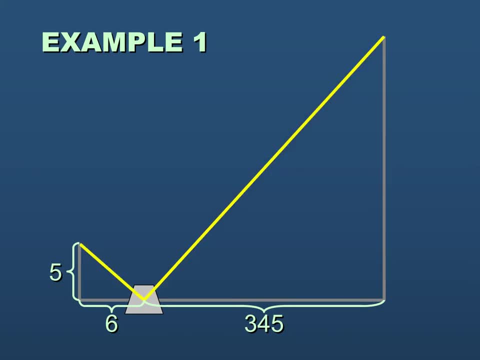 feet tall and we want to know how tall the building is. So, as you can see, there are two different triangles that are made and we know that those two triangles are similar to each other, Which means we can set up a proportion. We know that the height of the building over 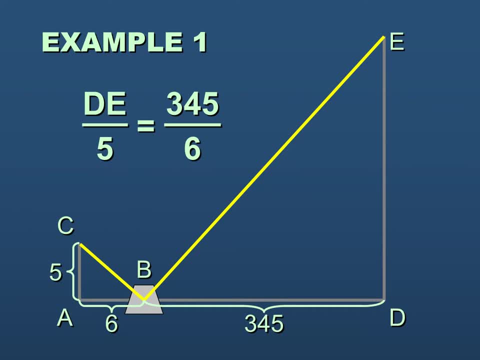 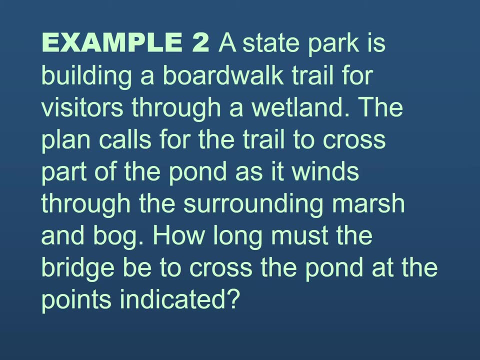 our height is equal to 345 over 6.. So we cross them and we can solve. And another example we have: a state park is building a boardwalk trail for visitors through a wetland, So the trail has to cross part of the pond. 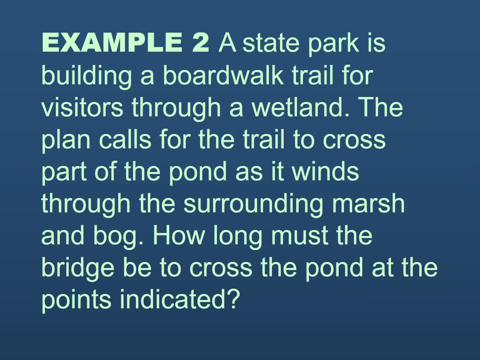 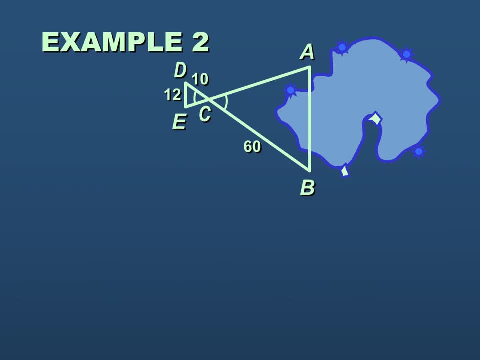 Okay, As it winds through the surrounding marsh. So we need to know how long must the bridge be to cross the pond at the points indicated? We have a diagram here. So what is the bridge right here over the marsh? We want to know. 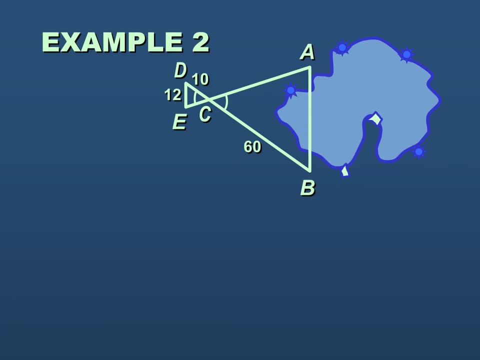 what the length is right here. So we know that these two triangles are similar, which means we can set up a proportion: This distance over this distance over here, and this distance over here Is equal to this distance over DC. So we plug in the information that we know. and now we? 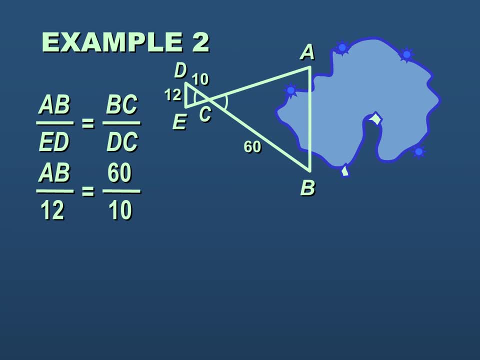 can cross. multiply to solve for the unknown. Okay, So divide both by 10, which means that the distance of the trail of the bridge is going to be 72 feet. Okay, So the distance over the park is significant and that is about 14,000 feet with the. measurement And looking in theे you can see that there is about 14 feet of distance in total. can used to called vertical line, So the distance is 0,000,000 miles. Dy.